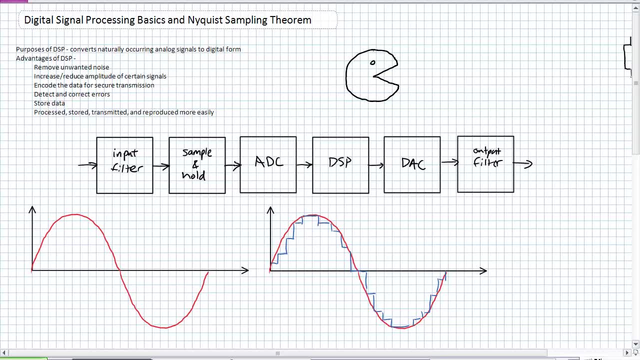 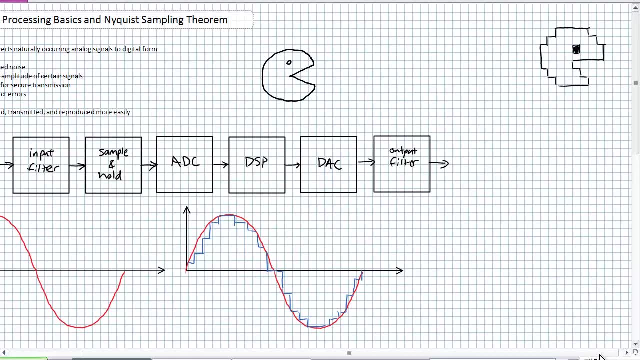 And the deal is, is that's not Pac-Man, That's your idealized representation of Pac-Man. Over here in my upper right hand corner of the screen is the actual Pac-Man as displayed by your 1980s era Atari or whatever game system. 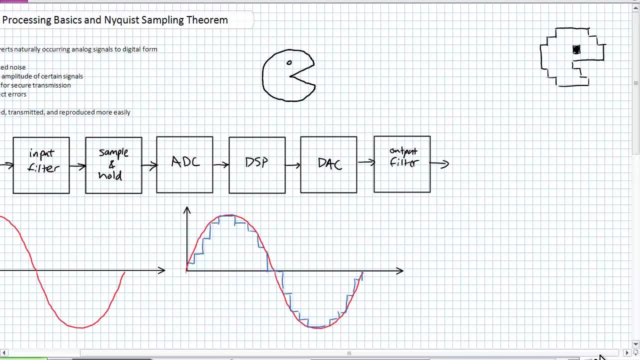 You know, notice how he's pixelated and blocky. However, it's close enough to round that your brain perceives him as such. You know, and that's the point of digital signal processing: It's to represent analog data As an approximated digital version, or vice versa. 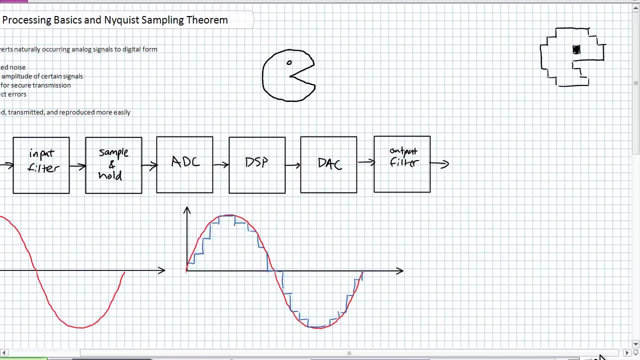 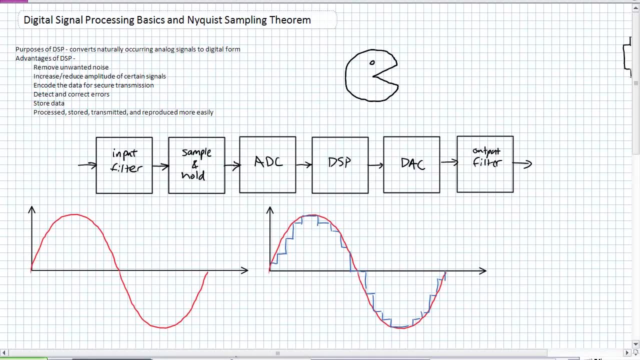 to represent digital data as an approximate representation of an analog signal, that it's close enough And the reason why we're doing this. there are certain advantages and they kind of go back to those beginning advantages. I talked about digital in the first place. 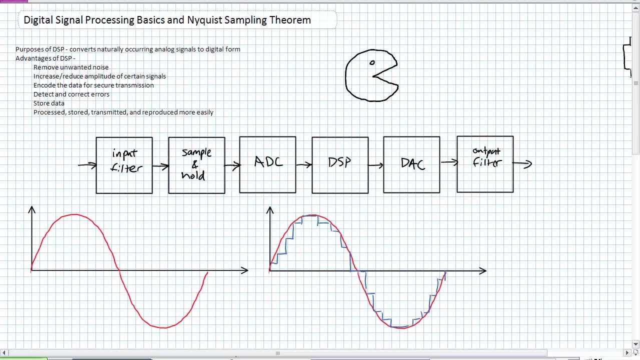 Okay, so the advantages of converting some naturally occurring analog signal to digital form: you could potentially remove unwanted noise. We could potentially increase or reduce the amplitude of certain signals. You can encode that digital data for secure transmission, Say, for example, a cell phone. 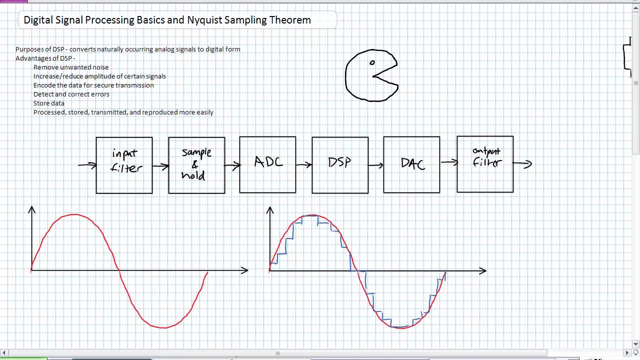 You can detect and correct errors. You could perhaps store that digital data a little bit better And, like I said, you're going right back to the very most basic lecture that I talked about in digital electronics in the first place. Why are we using digital in the first place? 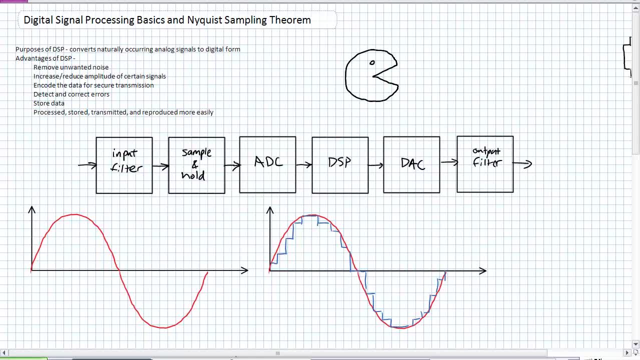 Because these basic advantages: it can be processed, stored, transmitted and reproduced more accurately and reliably and easily. That's the reason why we're taking this analog data, converting it to digital. in the first place, There is a certain basic block diagram to understand DSP. 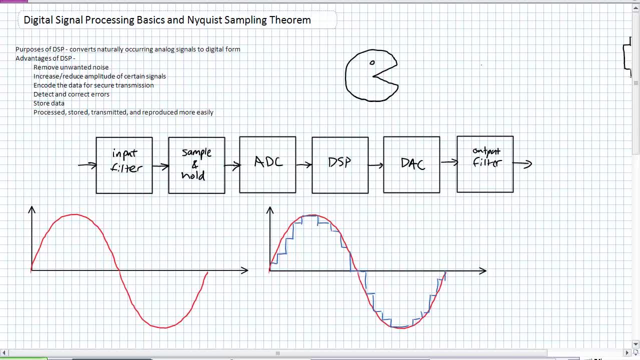 which I've got written right here. I've got a certain analog signal coming in on the left and it's being put into an input filter. So say, for example, there is this naturally occurring analog signal that has a spurious high frequency noise that you do not want included. 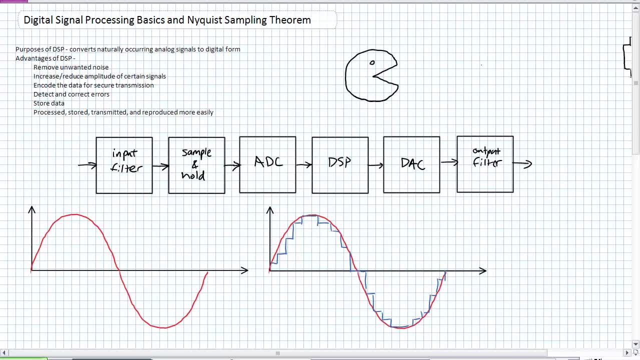 Say, for example, you would want to just go ahead and put in a low pass filter, get rid of that high frequency noise. So there's no sense including it in your data set if it's something you don't want to begin with. So there's this input filter getting rid of something. 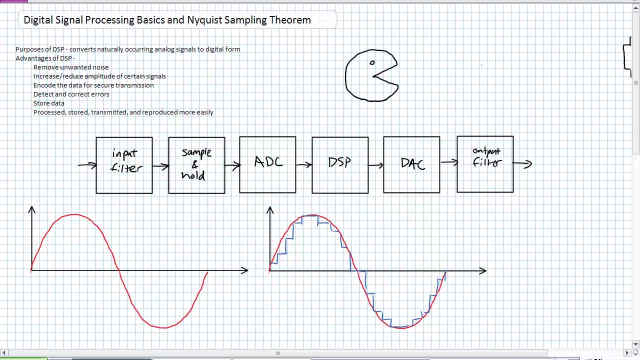 that you may not potentially want to include. This next block here is what's known as a sample and hold circuit. Okay, the sample and hold circuit is basically taking that smoothly varying analog signal which I've represented right here on the left-hand side with this red. 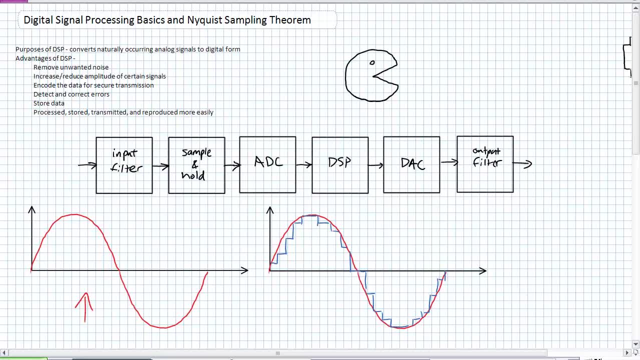 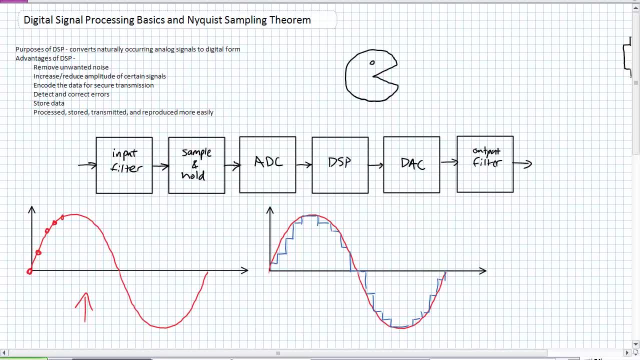 so on and so forth. basically, it is sampling at that point and it is holding it at that value until the next sample occurs, Because I know these things are smoothly changing over the period of time. however, there is a certain frequency at which we are sampling. 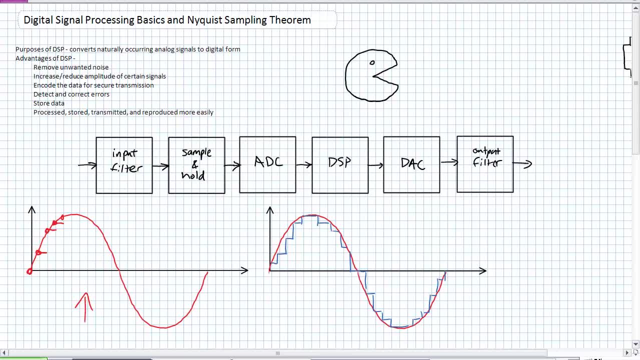 Okay, so it's sampling that data, holding it at the value it was sampled at until the next sample occurs, at which point it goes on to this thing called an ADC. This is really kind of the heart, or the first steps of digital signal processing. 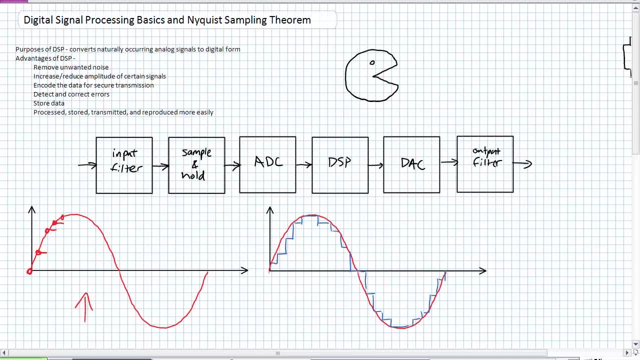 Okay, what is an ADC? It's an analog to digital converter. So ADC, analog to digital converter, And it's using that sampled positions and what it's doing it's quantizing it. So what does quantization means? It's basically, it's assigning binary value. 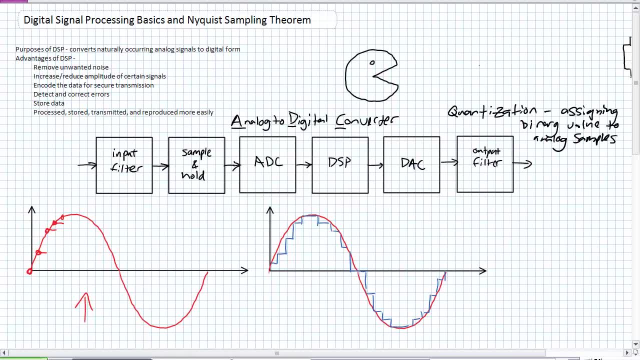 to those analog inputs. So again, quantization is basically assigning a binary value to those analog samples, And what I've drawn here on the right-hand side is a quantized representation of that same analog signal. So where we have given, these are supposed. 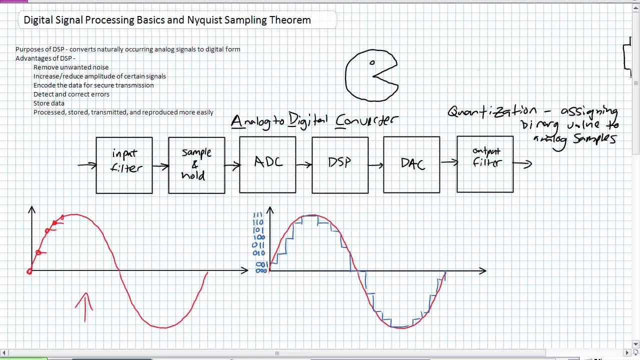 to represent binary values. Okay, these are supposed to represent binary values here. In our particular case, we've got a 3-bit quantization of that analog waveform. Let's see. For example, this is a- you know, a digital multimeter. 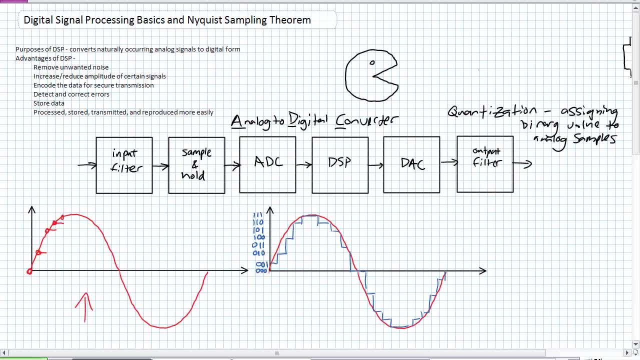 You know, it's sampling voltage levels smoothly, varying at certain periods of time, and it's assigning a binary value to each one of those, At which point this binary data is now being fed into this DSP. What is a DSP? It's a digital signal processor very similar. 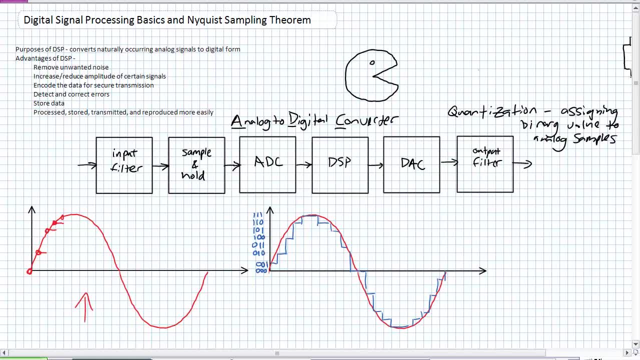 to a microprocessor, except it's handling some pretty advanced math at an incredibly, incredibly fast rate. I mean think about a varying, varying voltage signal Every 16.67 milliseconds. it's gone through its entire sequence from high- positive back to zero, to low negative back to zero. 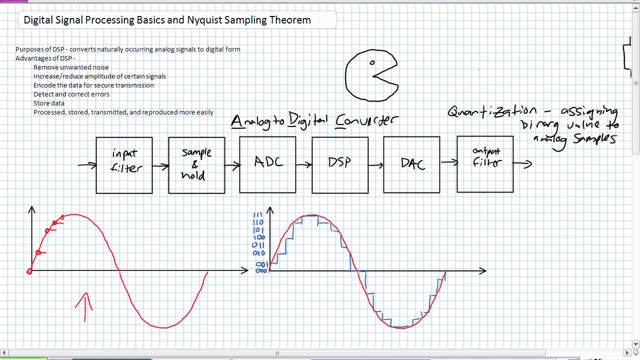 You've got to sample that at an incredibly fast rate. Think about speech, Think about music. All these things are occurring in real time. That digital signal processor is having to keep up with that. And what is that digital signal processor doing? Well, it's processing it, storing it, transmitting. 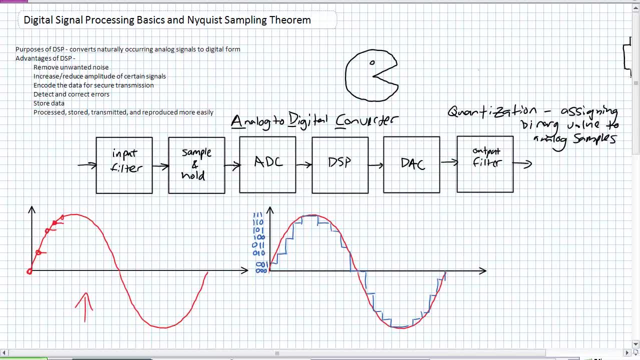 and or reproducing that analog data And, you know, removing that noise, basically all those advantages. That's what the digital signal processor is doing. It's going ahead and changing that binary representation of the analog data to a better form that might be used a little bit later. 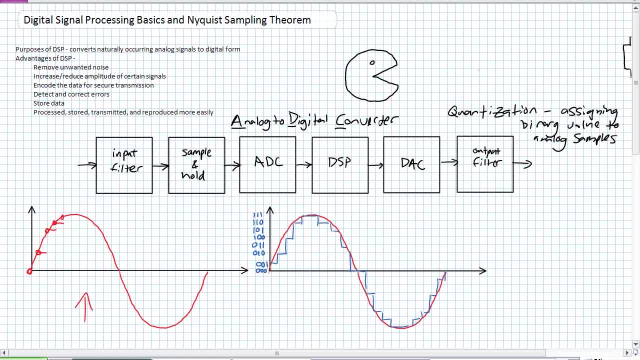 What is the next block in this diagram here? What's the DAC D-A-C? If A-D-C stands for analog to digital converter, what does D-A-C stand for? Obviously, it stands for digital to analog converter. digital to analog converter. 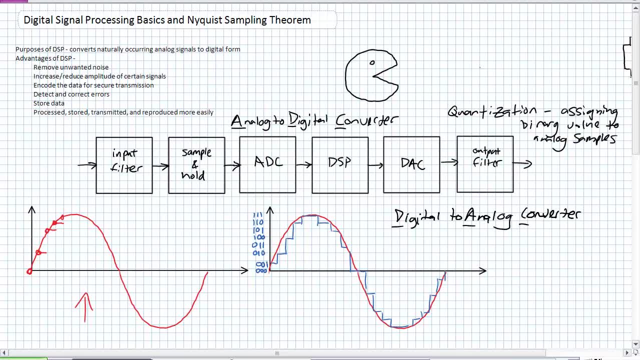 And that's basically what you're I think going to need, And that's basically what you're I think going to need, And that's basically what you're I think going to need. So a digital signal processor is kind of like your iPod. 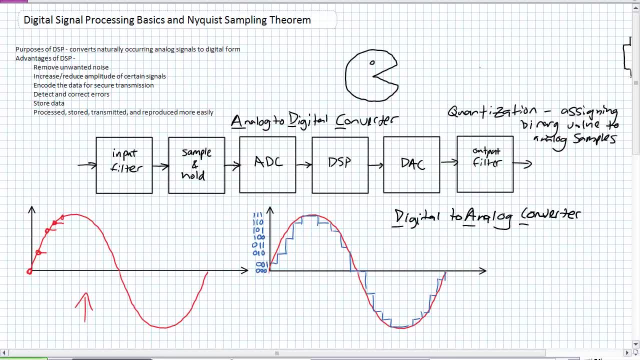 or your iPhone is doing to that digital representation of music stored on it? It's taking the digital representation, It's making an analog waveform which is being sent to the speakers. However, there might be an output filter, because notice the stair-step-like approximation. 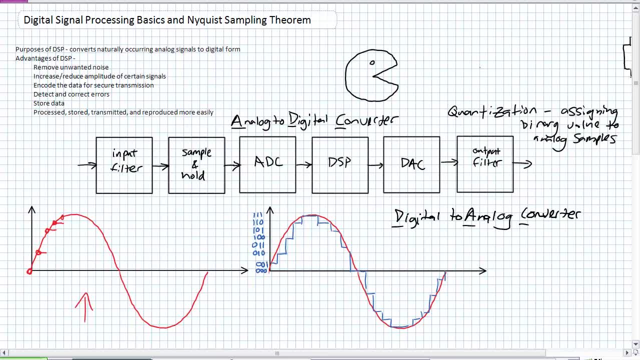 Our digital data looks like there. Perhaps we want to go ahead and smooth that output to a smoothly varying analog output which could perhaps represent music or speech or some other quantity. So this very basic parameter is going block diagram is going to be used over. 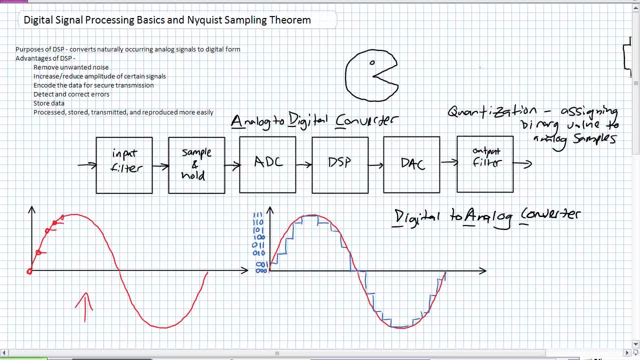 and over when we discuss DSP. We are going to go into in-depth ADC and the DAC and some of the methods used to go ahead and to do that, But your understanding of this basic step by step block diagram is pretty essential to your understanding of DSP. 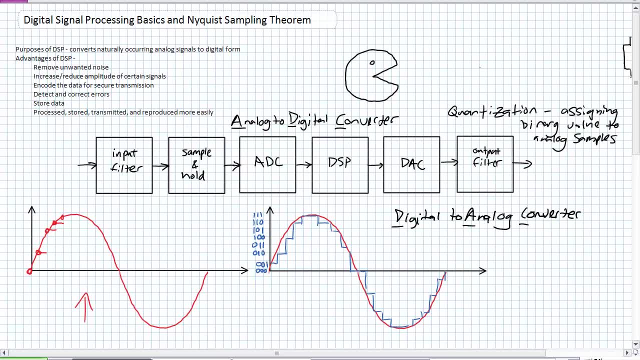 So I've only briefly mentioned this concept of sampling and frequencies, And I've also told you that, okay, I'm going to go ahead and forego the crazy math. All right, we do have to actually discuss some of the crazy math, and how we're going to do this is actually 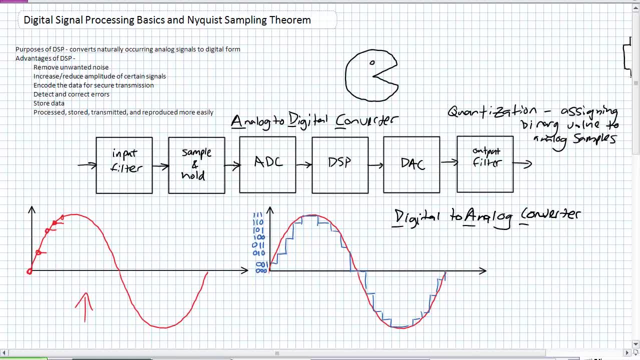 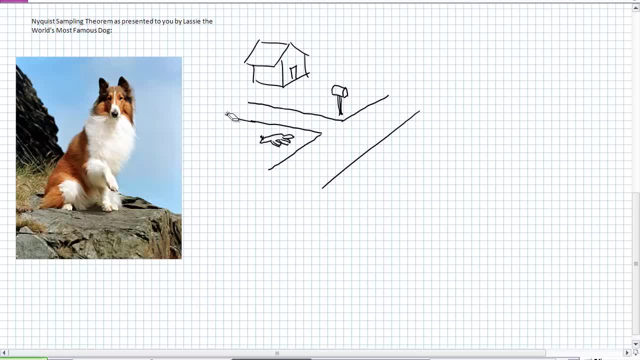 in a pretty easy method to discuss the Nyquist sampling theorem. So we're going to go ahead and discuss some pretty crazy, complicated math in the form of what's called the Nyquist sampling theorem, And we're going to have Lassie, the world's most famous dog, present it to you. 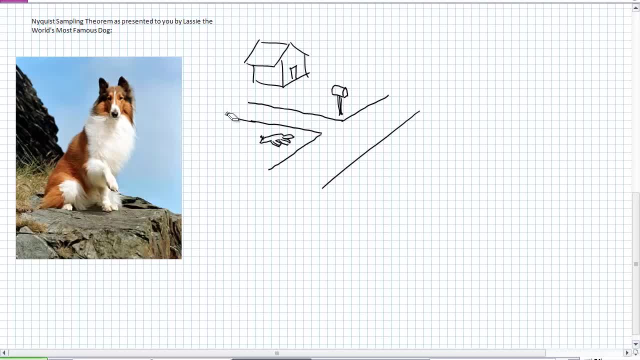 So to set up the joke here, what we've got is Lassie laying by the road asleep And Farmer Brown revs up his big old pickup truck and takes Lassie to sleep, He takes off for work and as he makes the turn going, 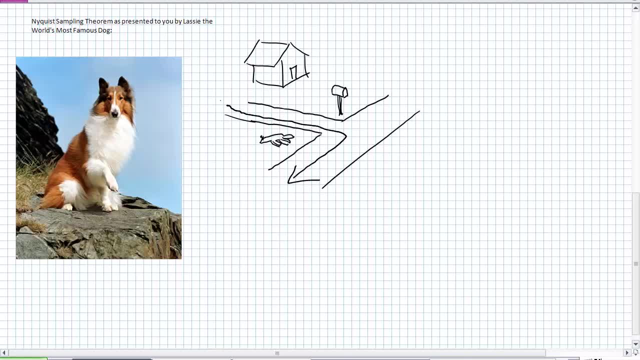 into town. he looks at Lassie and sees that she's asleep. Soon as the dust from Farmer Brown's pickup truck disappears over the hill, Timmy falls in a well. So what's Lassie do? Lassie responds to his cries. cries for help goes ahead. 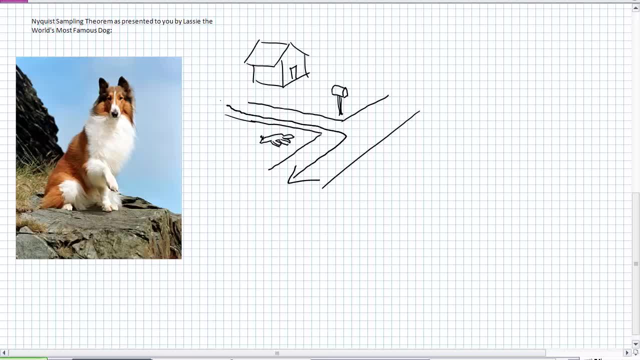 saves him, pulls him out of the well, gets him back inside the house. She lays back down and tries to get a nap. Two seconds go by Timmy's in the medicine cabinet. He's ingested a bunch of codeine. 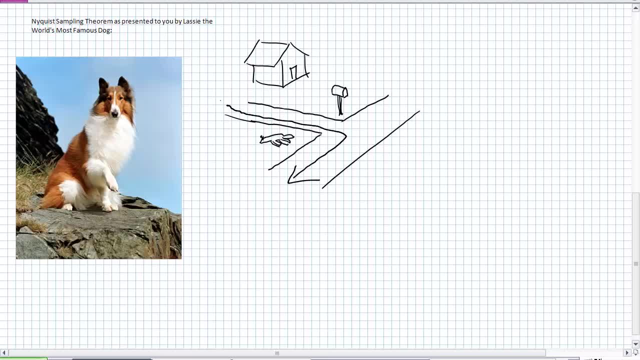 So Lassie's got to run inside, go ahead and get the codeine out of Billy And perhaps administer first aid, CPR, perhaps even use an AED. And now Timmy's doing fine. She puts him on the couch. 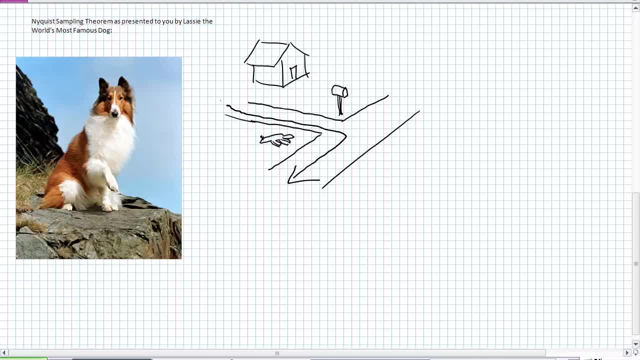 She goes back out, lays down, tries to take a nap. Pretty soon Timmy gets into the gun cabinet and he's shooting wildly in all different directions. Lassie goes ahead, calls the SWAT team, gets the SWAT team in there. they subdue Timmy. 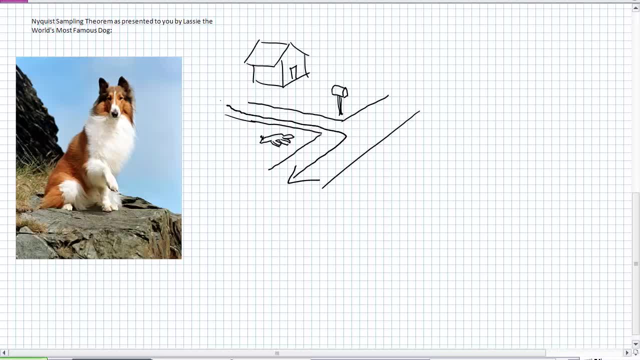 And then finally, Timmy's a little bit tired from today's activity, falls asleep. And then Lassie goes back out to the driveway and falls asleep again, At which point Farmer Brown comes back from work. He's making a turn into the driveway. 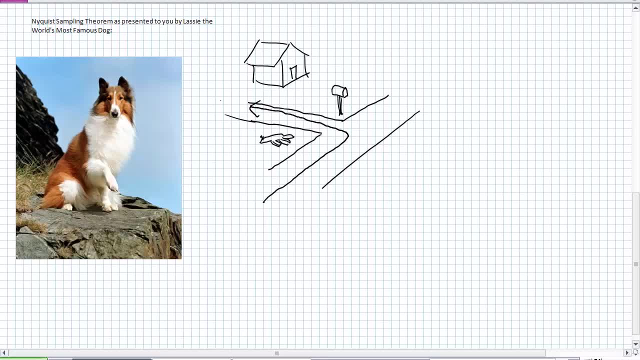 He sees Lassie asleep by the driveway. He looks at her and he says: lazy dog. Point of that joke is Farmer Brown did not sample Lassie at the correct frequency. He only looked at her two times during that day. She happened to be in the same position. 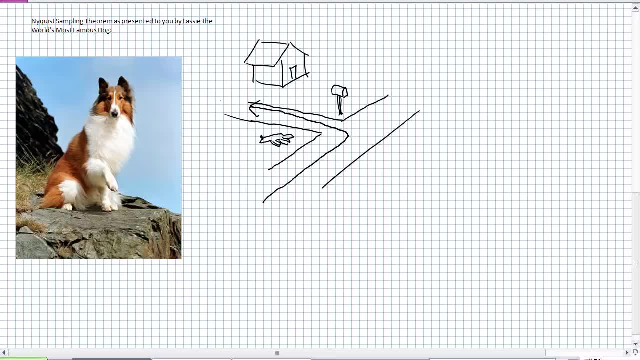 So what this Nyquist sampling theorem states is: you've got to go ahead and sample something at least twice the frequency at which it is naturally occurring, And had Farmer Brown not done that, Farmer Brown wouldn't have been there more than two times during the day. 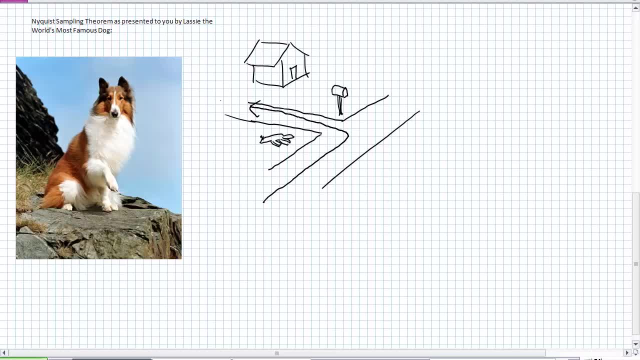 He would have realized that Lassie had in a pretty, incredibly difficult day. And that's the point of the Nyquist sampling theorem. You're going to go ahead and have to sample a naturally occurring analog piece of data at twice the frequency that you wish to capture, to go ahead. 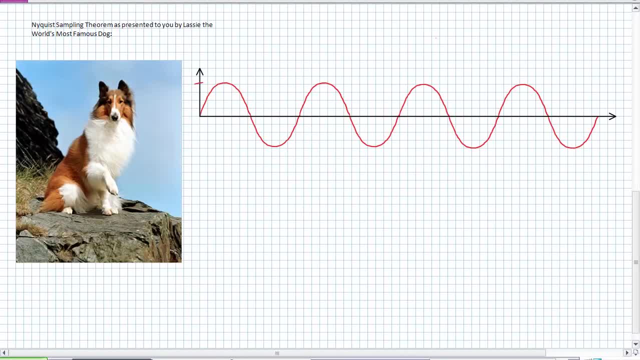 and reliably reproduce that data And a simple illustration of the Nyquist sampling theorem gone terribly wrong. Let's use the Farmer Brown method Here. what we've got is an analog signal of a certain frequency. Let's say it is a United States distribution wave. 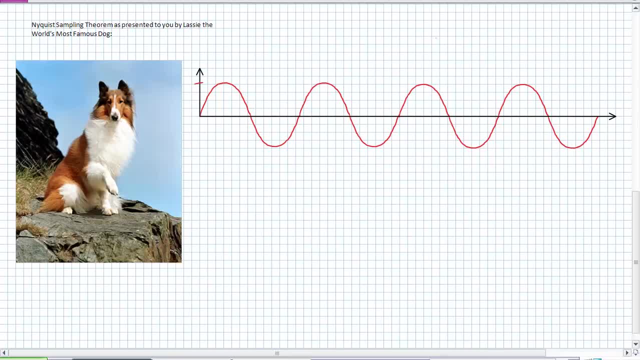 So it's 60 hertz And let's sample it at 60 hertz. Okay, Let's say our first sample occurs here, The next sample occurs here, here, here, And because we are inappropriately sampling this at an inappropriate frequency, very clear, you're like oh, 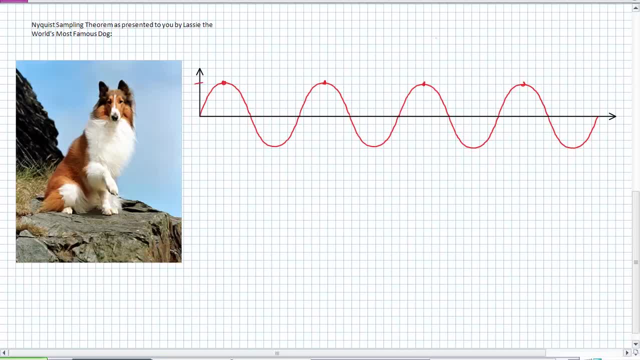 it's obviously a 170 volt DC signal. You get the point here Is it is not a DC signal. It's a DC signal at 170 volts constantly, Because it is taking a value from 0 to positive 170, back to 0, down to negative 170, with an RMS value of 120 volts. 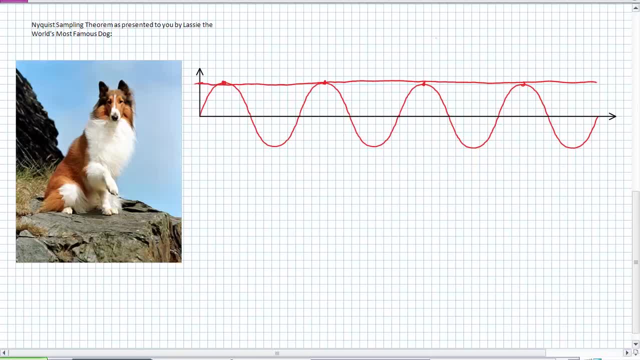 So that is a misapplication of the Nyquist sampling theorem, Very clearly demonstrating that it is being aliased. You know, think about an alias. You're it is a disguise. Okay, It is not a DC signal, It's in fact an AC signal. 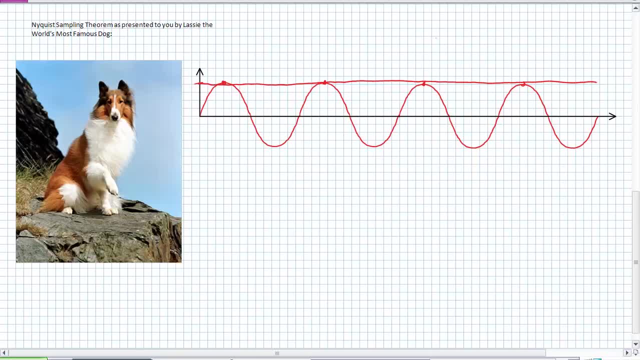 And this misapplication. you know this Farmer-Brown method of just looking at it not with the correct frequency, you're going to get all sorts of bad values. Let's just say, for example: our first sample is right there. 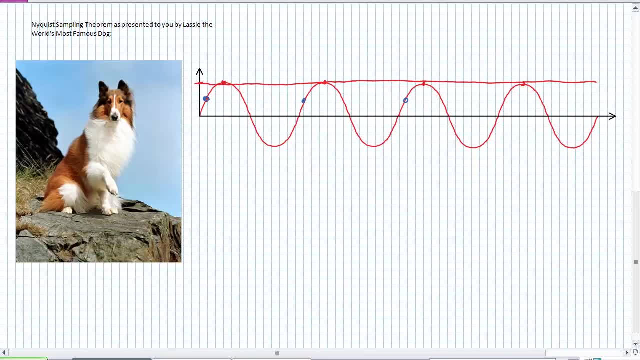 Let's do that. one in blue. Our first sample is right there, right there, right there. If you're occurring at that 60 hertz frequency, you're going to say, okay, it is obviously a certain DC value And it's not. 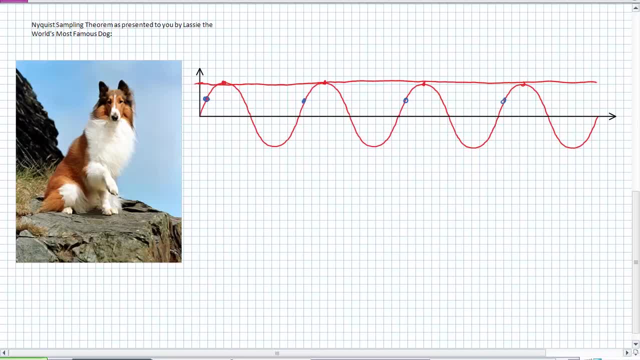 Okay, So you're incorrectly sampling this thing. The Nyquist sampling theorem is: we're going to have to have to. when we sample this wave, in this particular example, at 60 hertz, we're going to have to sample it at 120 hertz. 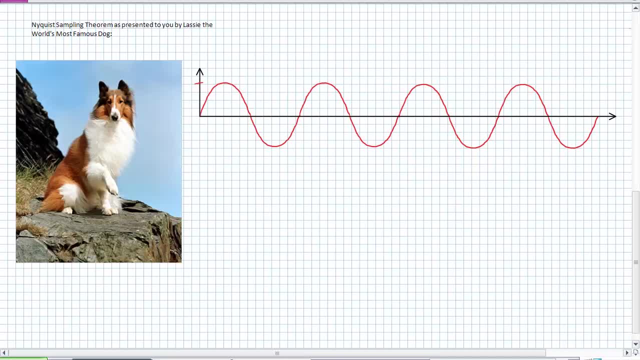 to accurately represent this wave. So the naturally occurring period of this is right there for a single cycle. So let's say we sampled there and there. What we're getting is a positive maximum and a negative maximum. It is not exactly the prettiest rendition you know of a wave. 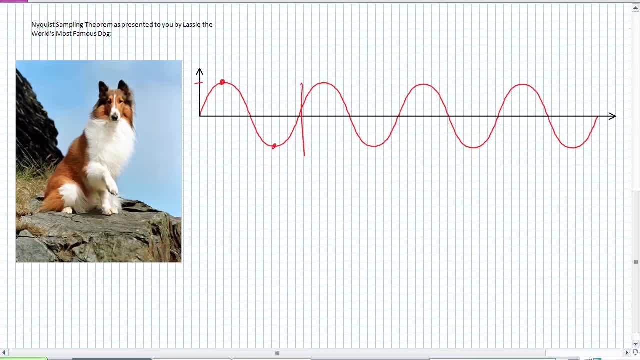 But if we know that we are sampling a sine wave to begin with, we can accurately recreate that sine wave, knowing that it peaks out at a certain value and bellies out at another negative value. There are advantages perhaps of sampling at an increased frequency. 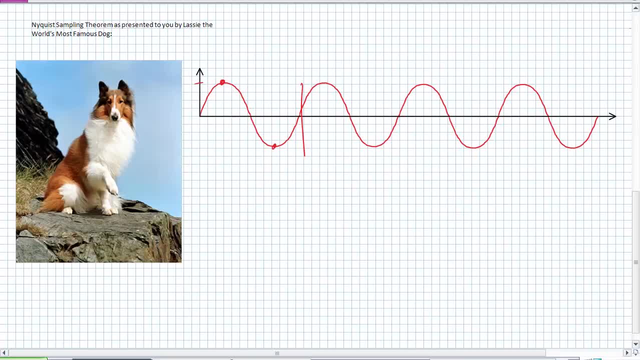 because you could potentially gain better representation of it. but we're not necessarily always sampling just a pure sine wave, and this is where the crazy, crazy, crazy math comes in, And I do want to illustrate a little bit about some of this crazy math here. 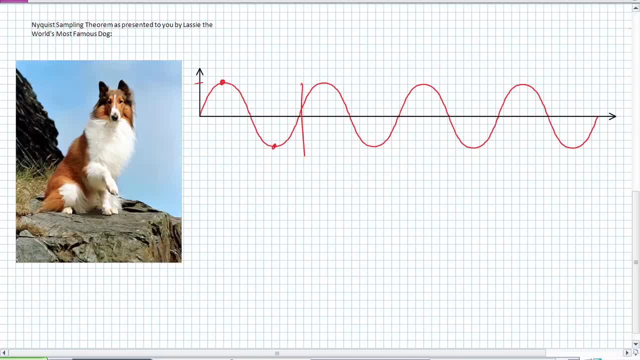 And I'm going to start off with this basic statement, which may surprise you: Everything is sine waves. Every piece of information that can be, any signal, is a summation of sine waves, including digital pulses. okay, And this is crazy, And even to the point of reality, you know. 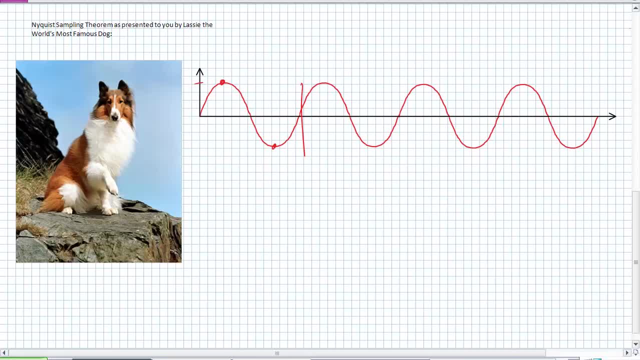 because one of the most famous quotes from Nikola Tesla is: if you want to find the secrets of the universe, think in terms of energy frequency and vibration Reality. as we get down to it, we are finding that, as we get smaller and smaller, we're realizing nothing's there. 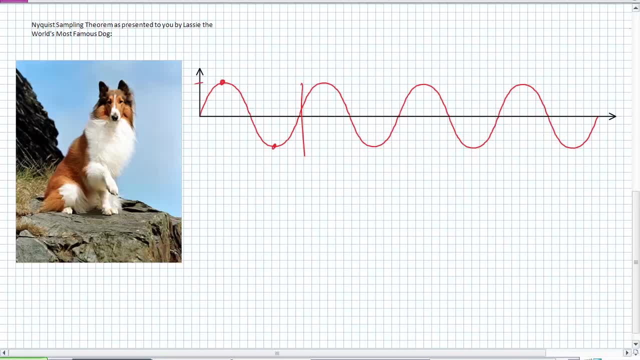 but vibrations and frequency okay. So that is crazy, crazy math. What I want to talk to you here is just how you can possibly create summations of sine wave, And one of the simplest ways to do this is take your TI-89 graphing calculator. 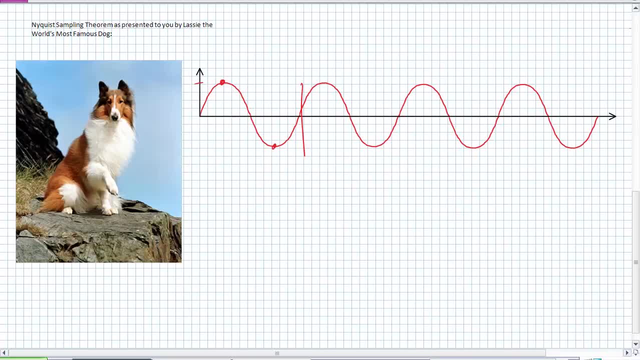 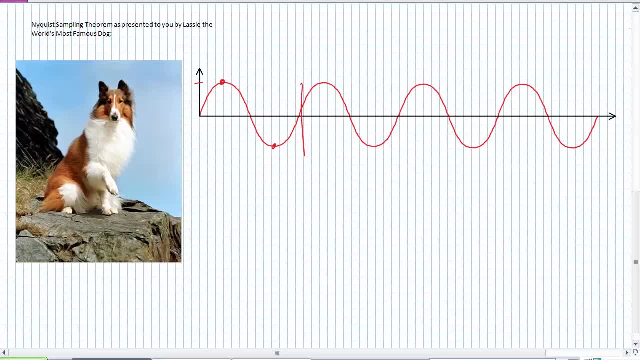 They're called sine waves. They're called sine waves. They are different analog values, but they are composed of sine waves, And one of the ways I want to do this is a pretty crazy example- is a digital pulse. How can I represent a digital pulse? 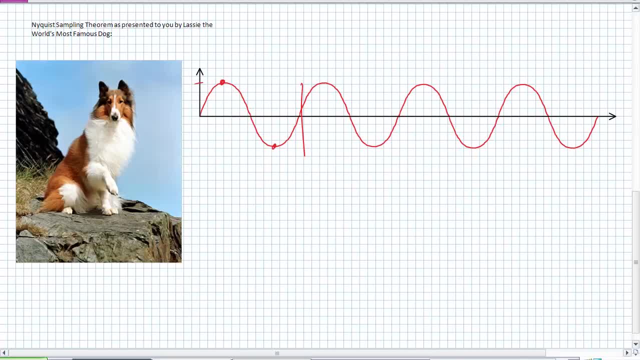 as a summation of sine waves. Well, let me go ahead and just draw some diagrams here. So look at this digital pulse here It's not a sine wave. How can I use sine waves of different frequencies to go ahead and represent this digital pulse? 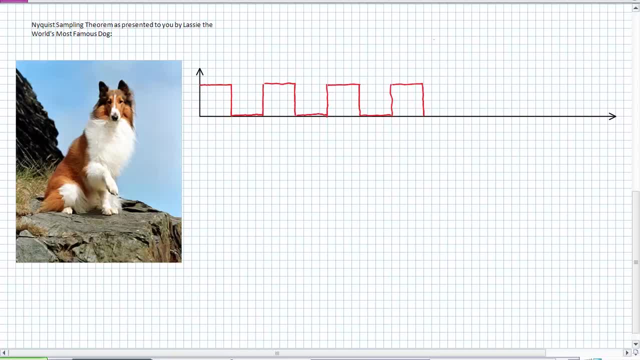 Well, first off, what I'm going to have to do is just think about a sine wave. It's zero centered, This is not zero centered. I'm going to have to raise it up by a certain amount. Okay, so there's this DC component in this. 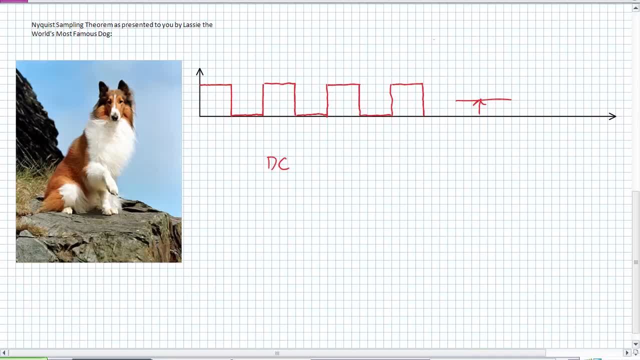 So this idealized representation of this digital- excuse me, the summated sine waves representation of this digital pulse, There is a DC component plus some sine waves And those sine waves have a magnitude of a certain value and amplitude and frequency. The more sine waves you put into this, 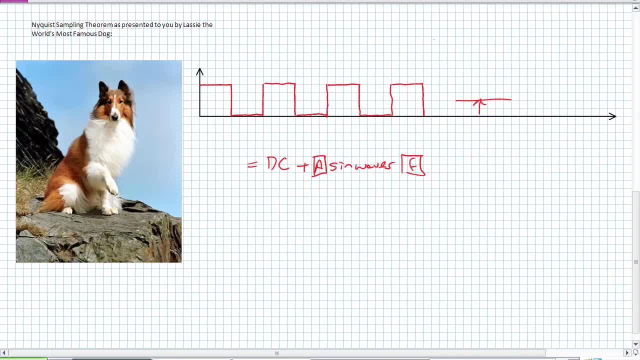 the more you can accurately represent any data. So I've chosen the digital pulse because it's one of the hardest things for you to do to realize that, okay, sine waves can be used to create anything. If we've got a bias, we've got a DC bias here. let's just say: 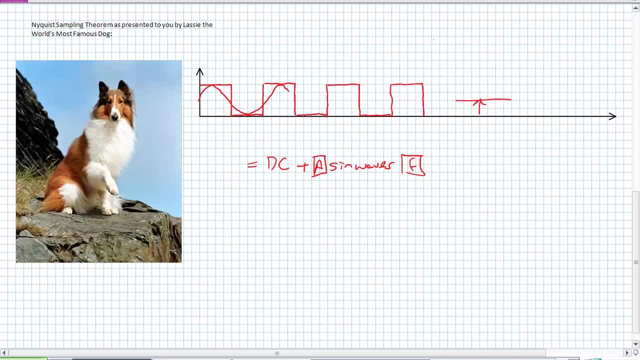 if I took a sine wave of the fundamental frequency- let's say again, it's 60 hertz- That kind of looks like a digital pulse, It's not you know, but it's a little bit closer And that is a certain amplitude which I'm going to call 1.. 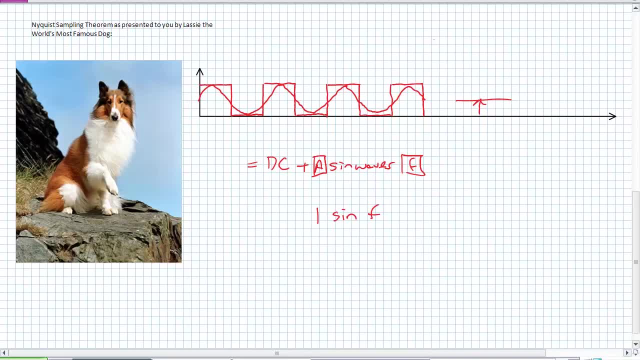 One sine of the fundamental frequency. What if I added to that? So I've got my DC component, I've got amplitude 1 of the fundamental frequency. What if I added the following: One-third of sine 3f. What is one-third sine 3f? 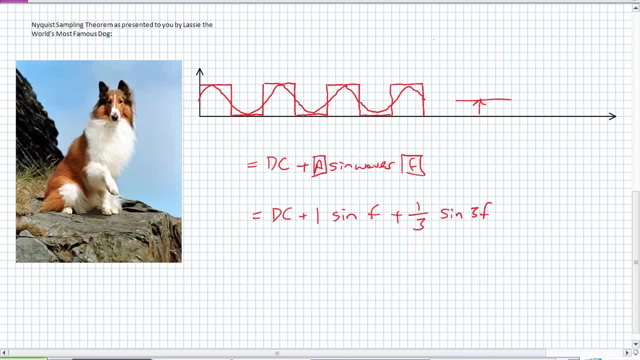 Three times the fundamental frequency, but a third of the value. Well, think about it. If this is the full period with an amplitude of 1, what is one-third of that? Well, it's obviously going to be maxing out and minimizing. 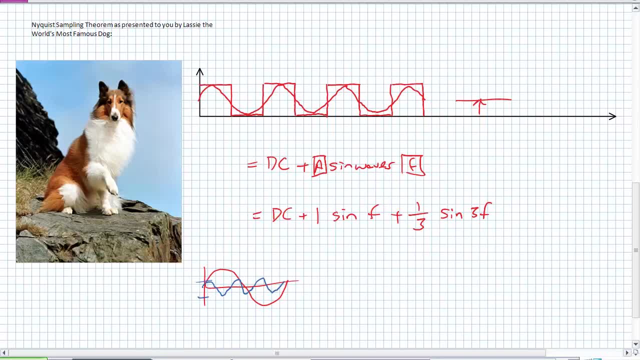 out one-third of it, But it's going to go through three full cycles in that same period And when you add one-third sine- 3 times the frequency to one sine, one frequency- believe it or not- what you're getting is kind of something like this: 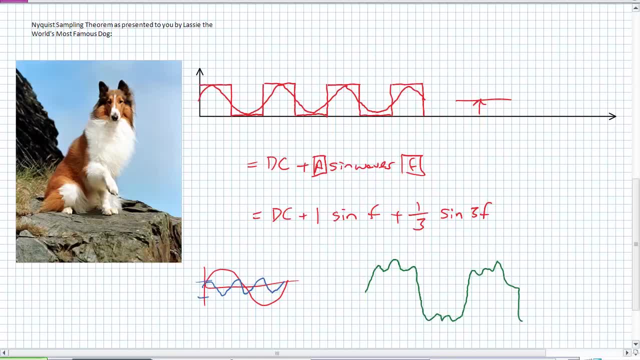 Does that look a little bit more pulse-like to you- And I know I'm messing it up, Like I said, waving my hands at certain things here And now continue to add components. One-fifth, sine of 5 frequency, That summation of that DC component. 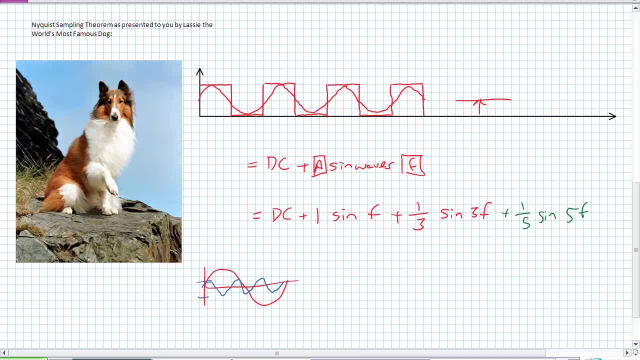 the fundamental frequency. three times the frequency, five times the frequency, What you're getting is a fundamental frequency and you're getting a little bit closer to that pulse. Add seven times, You're still going to get a little bit of an overshoot and ringing there. 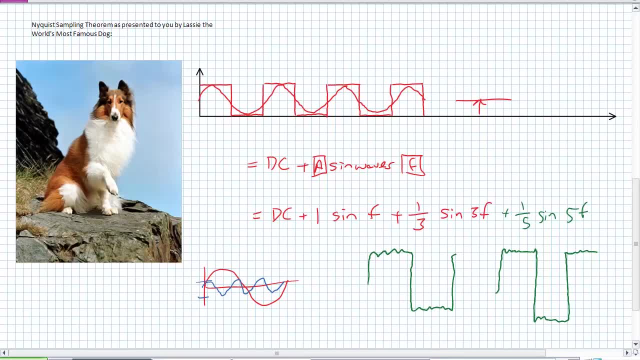 You're going to get closer and closer. This is the point. what I'm trying to say is: everything is sine waves. And now, when I say that, the Nyquist sampling theorem, you have to do two times the highest frequency which you can't wish to capture, how accurately do you wish? 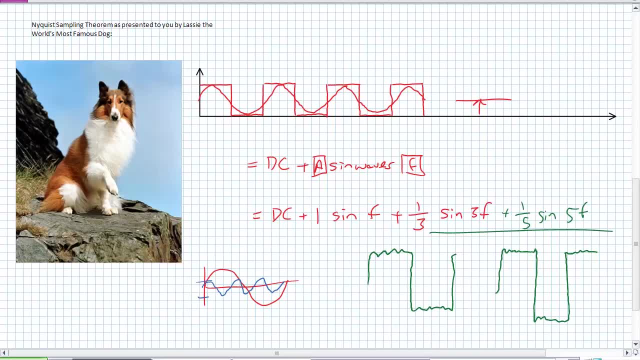 to capture this digital pulse data, Because this thing goes on forever. And this is what I'm saying about. there's some creativity, There's some crazy math here. Don't worry about the crazy math, but realize that everything is a summation of sine waves. 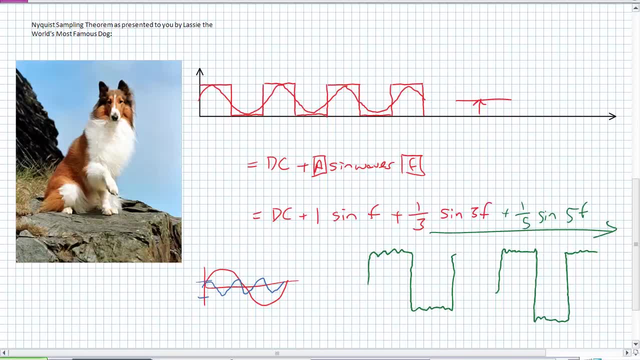 I would have to go on forever and my to accurately, truly represent clear digital pulse. However, can I go twice the frequency of forever? No, the answer is no, you can't. There's a practical limitation to these. So you're going to get a idealized representation. 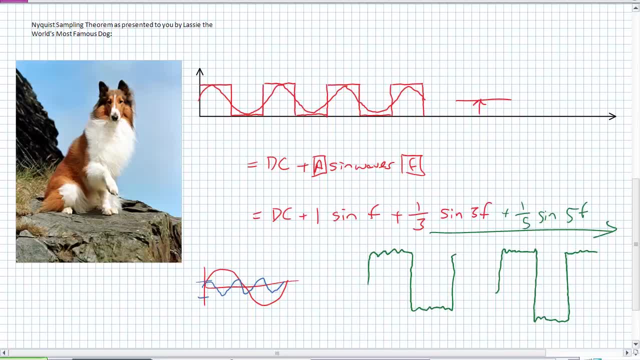 Your Pac-Man can never be the truly analog version of Pac-Man, but it can get pretty darn close. Now that I've done an incredibly complicated example, you should realize that everything can be presented as sine waves, You know. think about the audible range for human speech. There's a certain frequency low and a frequency high that can occur. Why would you ever sample something out of that range if it's not going to be heard to begin with? We've got this range right here and do not quote these things. 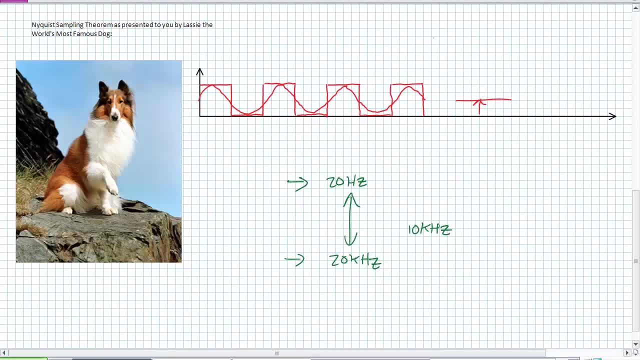 These things are. I'm just doing these things off the top of my head here. If I remember right, like the human hearing response is around 20 hertz. if I remember right, maybe even lower 6 or 8 hertz, up to 20 kilohertz. 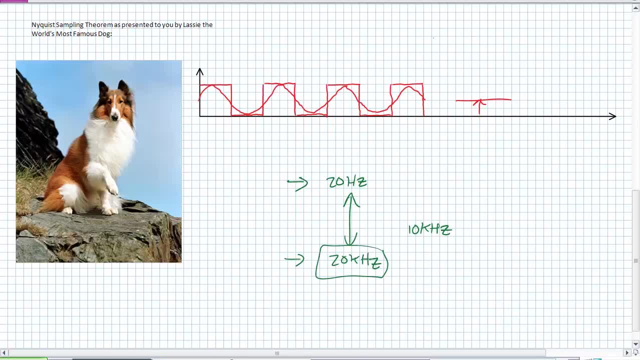 That's human hearing response range And this 20 kilohertz maximum here is really kind of representative of your age, Those individuals that with younger ages. I do this experiment in my electronics one class. I get something going at 22 kilohertz and I slowly drop it. 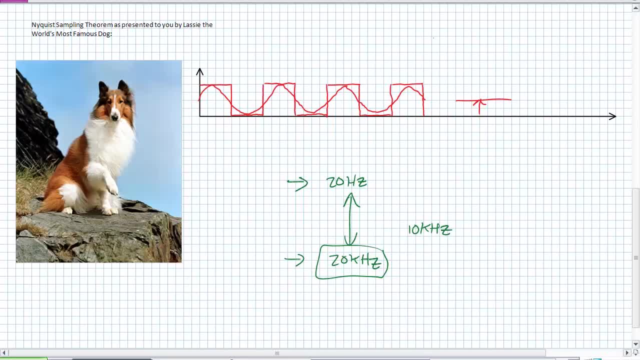 Down, and I see which people turn their heads to hear the noise. first, and it's always the younger students that do so. Okay, And then pretty soon, I'm lowering it down, lowering it down, lowering it down, and finally some of the older students. hey, I can finally hear that. Okay, so that upper range might be around 21,. 22 kilohertz, Most people 16 kilohertz. you know you're going to hear that. So the point is, is the human hearing range goes from that 20? 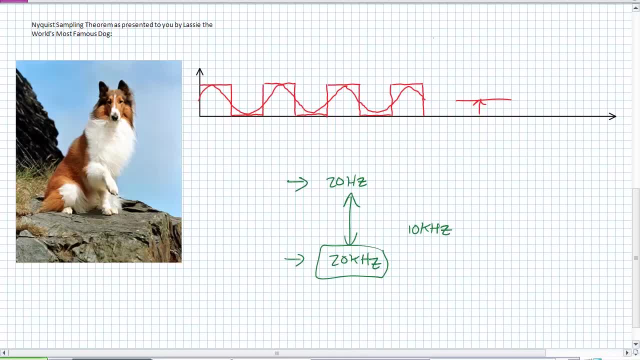 to 20 kilohertz. for our purposes of this example, However, human speech kind of tops out at 10 kilohertz. You are potentially just talking. You're not playing a musical instrument, You're not doing anything like that. You know what is the minimum frequency? which would you be? 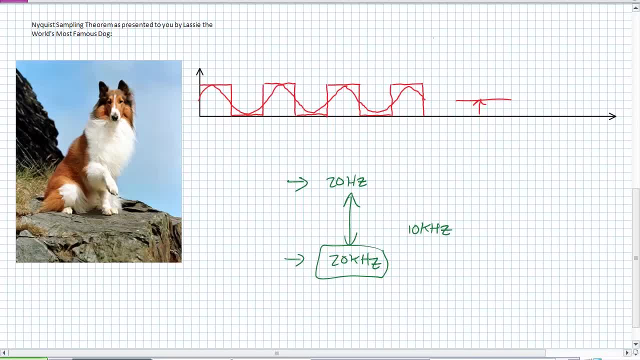 sampling which you should be sampling human speech at. The answer is is twice its maximum, so it's 20 kilohertz. So if I wanted to do very, very accurate representation of, well, reasonably accurate representation of human speech, 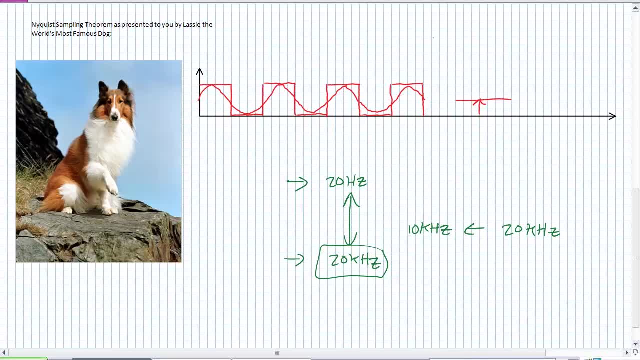 I want to sample it at 20 kilohertz, That waveform that you know, it's obviously not a pulsed waveform, But it is a waveform, you know, of human speech And like I said previously is I know that's not a pure sine. 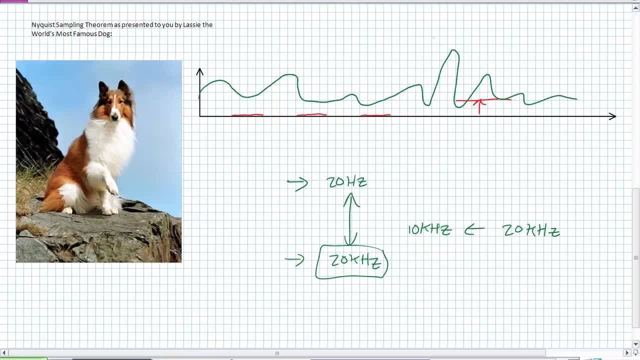 wave, but it can be represented as a summation of sine waves, The highest frequency of which is around 10 kilohertz for human speech. I don't mean to delve into the crazy esoteric math too much here, but it is important for you. 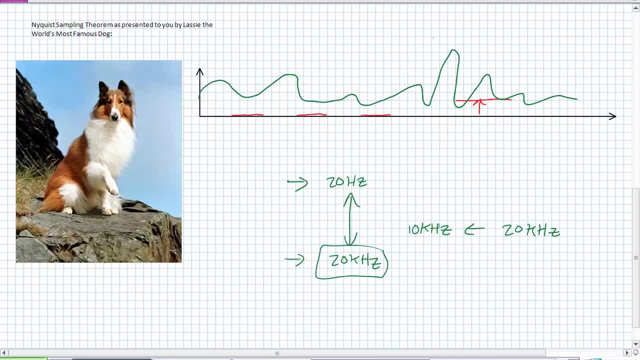 to understand. pretty much everything can be composed of sine waves And for you to accurately represent it, there is a certain frequency which you want to and you're going to go ahead and somehow neglect certain amounts of data which may not be necessary for your accurate representation later on. 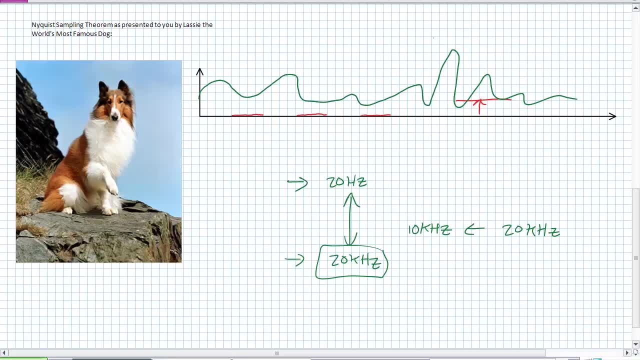 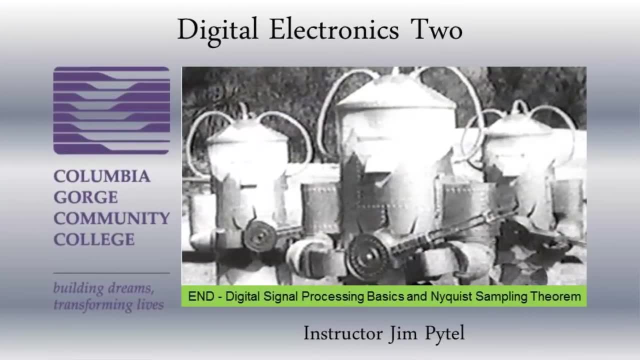 So this concludes the lecture: digital signal process and basics. and nice, with sampling theorem We're going to go into converting analog signals to digital, basically the analog to digital converter.